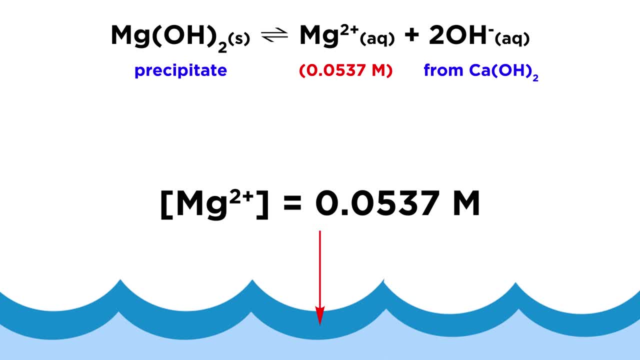 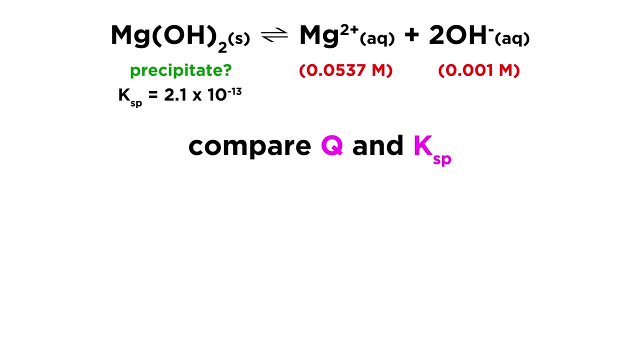 and let's say we want to find out if enough calcium hydroxide is added to give a hydroxide concentration of 0.001 molar, will magnesium hydroxide precipitate form, Given that it has a KSP of 2.1 times 10 to the negative 13.? 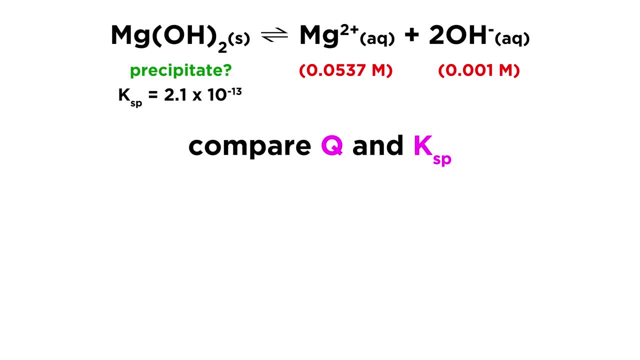 As we said, we simply need to compare Q and KSP. so let's calculate the reaction quotient Q. If Q is equal to magnesium ion concentration times hydroxide ion concentration squared, then plugging in those concentrations will give us a reaction quotient of 5.4 times 10. 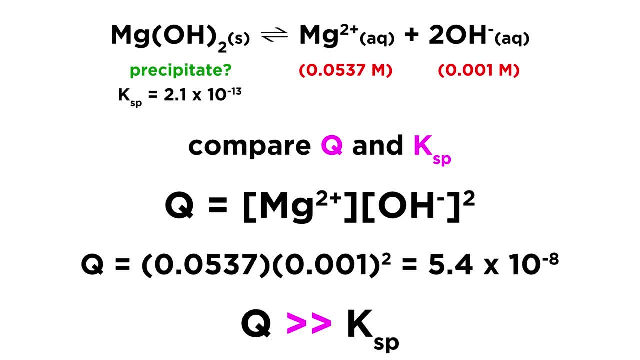 to the negative 8. This is significantly larger than KSP, And we know that if Q is greater than KSP, then the reaction quotient will be greater than KSP. If Q is greater than K for any type of equilibrium, the equilibrium will shift left. in this case, 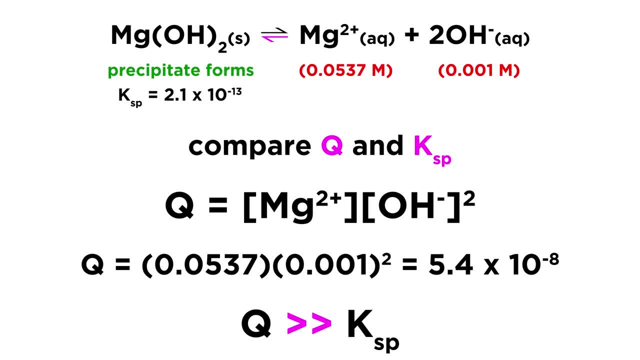 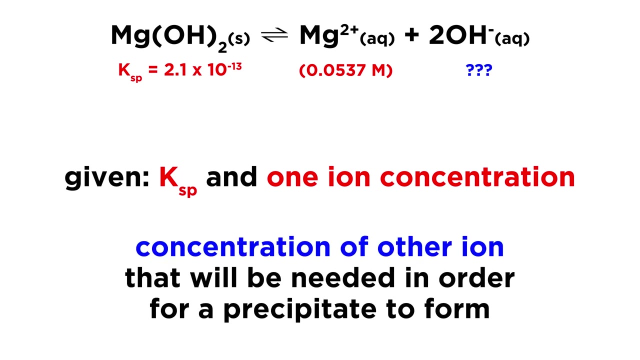 producing solid. thus, precipitate will form until Q becomes equal to KSP. If we consider a similar situation where the only difference is that Q is less than KSP, a precipitation will not occur and all ions will remain in solution. This also means that, given a KSP and one ion concentration, we can calculate the concentration. 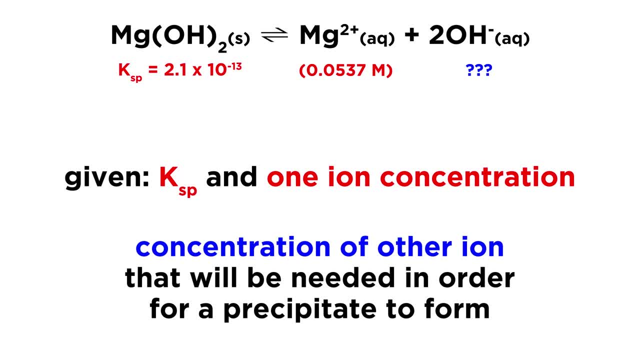 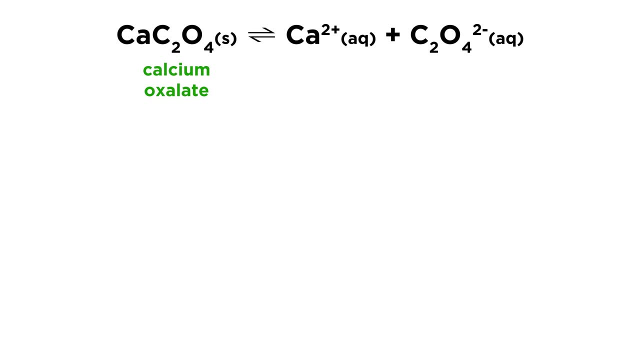 the other ion will need to reach in order for precipitation to begin to happen. We just need to find the concentration at which Q will become equal to KSP, For example. look at calcium oxalate. This substance can be in equilibrium with the calcium ion and oxalate ion, and it has 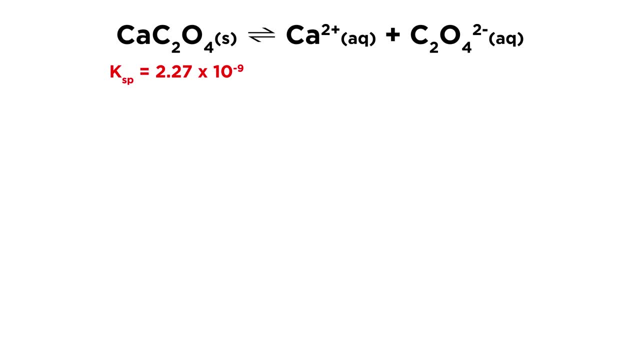 a KSP of 2.27 times 10 to the negative 9.. If we have a solution of this substance that is completely dissociated and the concentration is equal to KSP, then we can calculate the concentration at which Q will become equal. 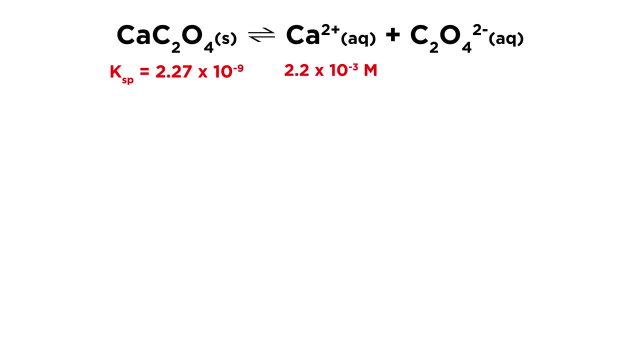 to KSP and the concentration of calcium is 2.2 times 10 to the negative 3 moles per liter. what must the oxalate ion concentration climb to in order for precipitation to occur? Once again, precipitation occurs when Q equals KSP, so we can simply write out the KSP expression. 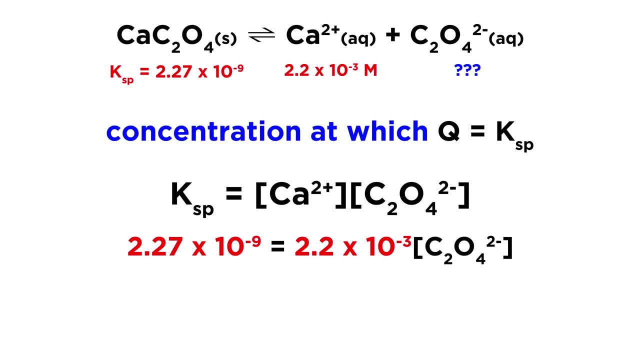 and plug in the two known values, that would be the KSP itself and the calcium ion concentration, Solving for oxalate concentration, We get 1 times 10 to the negative 6 moles per liter, which is the necessary oxalate. 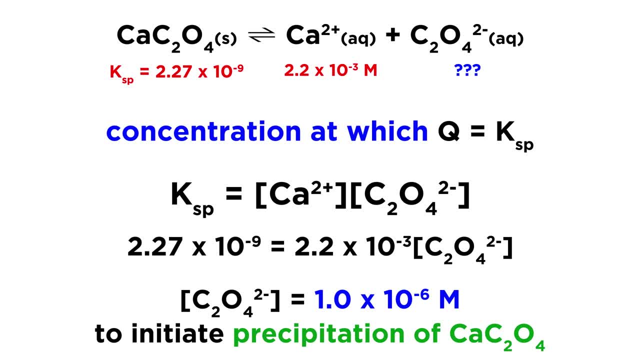 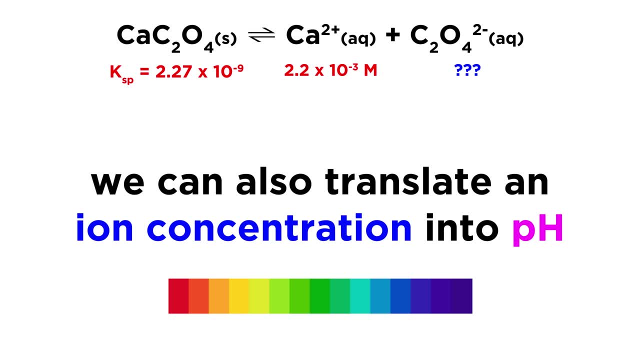 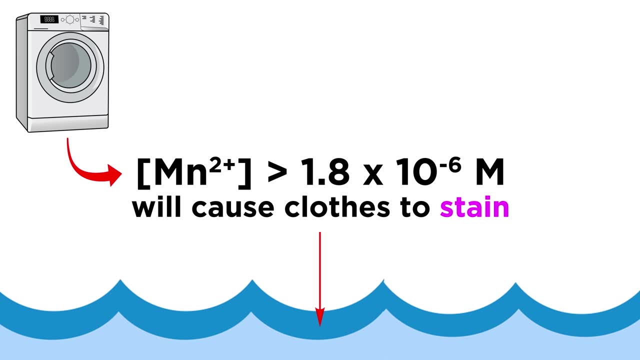 concentration to initiate precipitation of calcium oxalate. This concept can be modified to translate an ion concentration into a pH when acidity and basicity are concerned. An application of this is that water with a manganese ion concentration above 1.8 times 10 to the negative 6 moles per liter will stain clothing when doing laundry, which is why 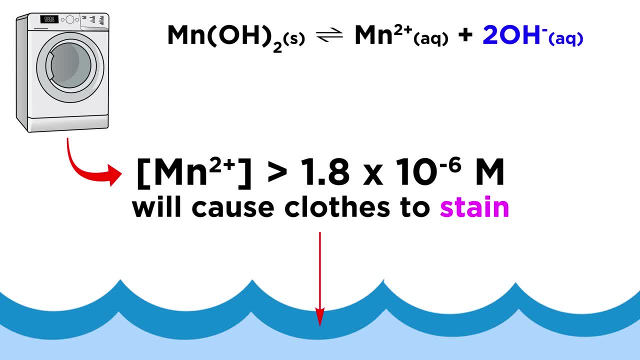 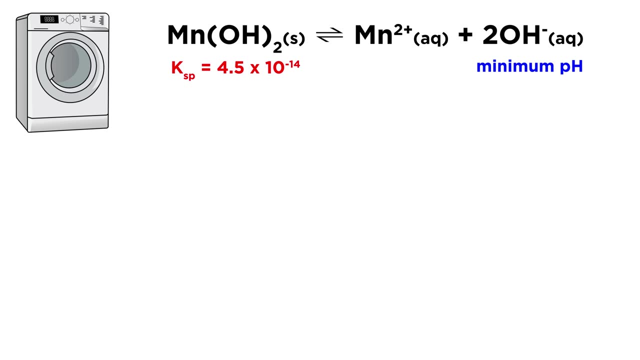 manganese concentration is sometimes reduced by adding base. If the pH is maintained above a certain level, the manganese can precipitate as manganese hydroxide and will thus be unable to stain the clothing. So, given that this substance has a KSP of 4.5 times 10 to the negative 14,, what pH is? 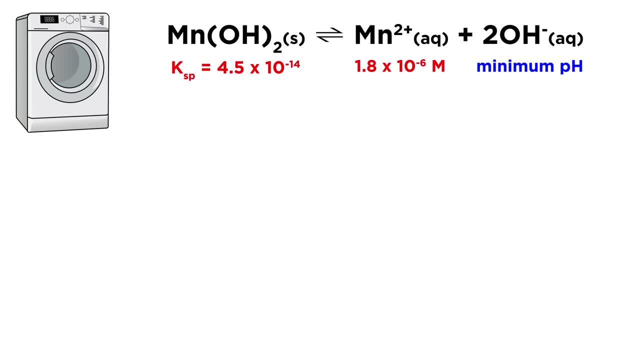 required to provide enough hydroxide to keep the manganese concentration at or below 1.8 times 10 to the negative 6 moles per liter. We use the same process as before. We are looking at the point where precipitation occurs, so we can just write out the KSP expression. 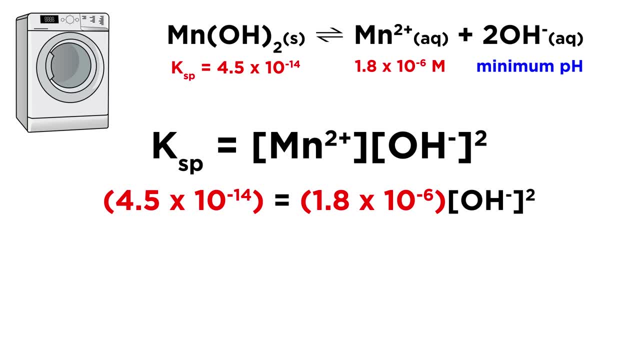 and plug in the KSP and the manganese concentration we are interested in. This will allow us to solve for the hydroxide concentration, which will be 1.6 times 10 to the negative 4.. From this we take the negative log to get the pOH and then subtract from 14 to get 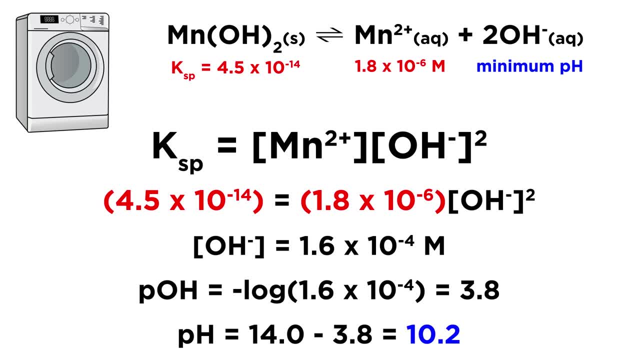 the pH, Which will be 10.2.. Therefore, if there is enough base in the detergent to keep the pH above 10.2, the manganese ion concentration will remain below a threshold that would stain the clothes. And that illustrates just a few applications of the solubility product. 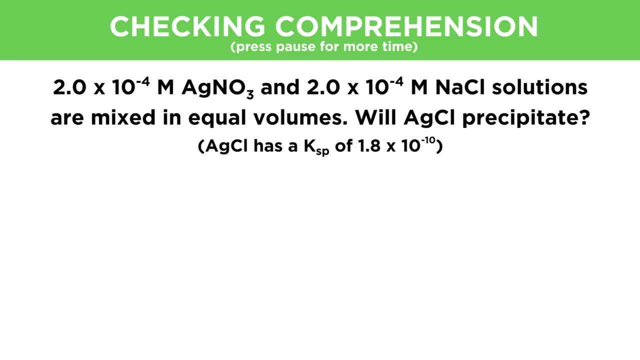 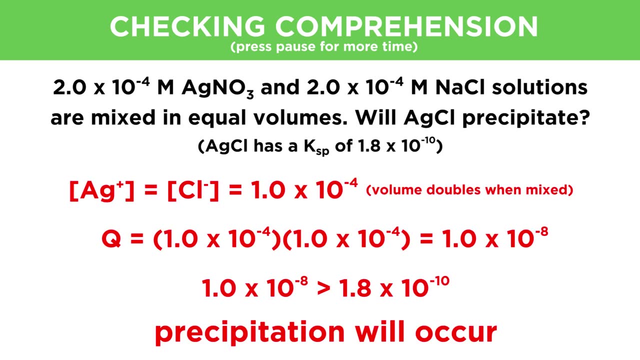 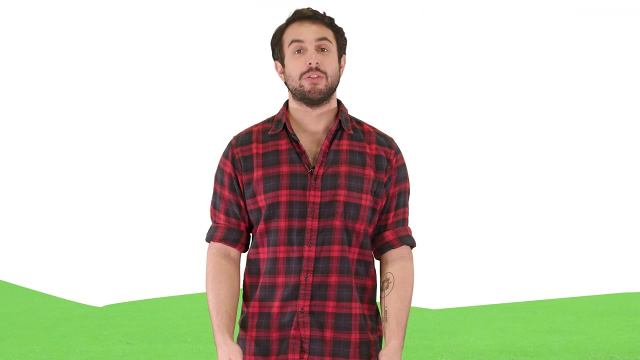 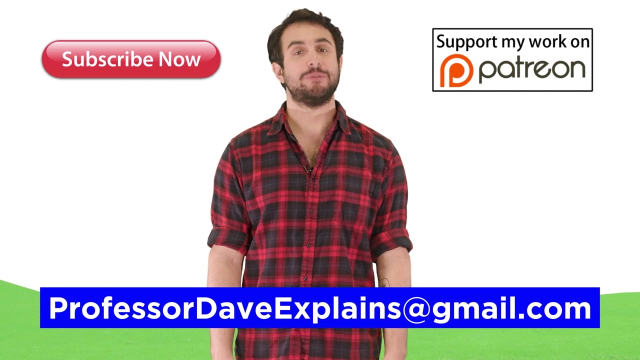 Let's check comprehension. Thanks for watching, guys. subscribe to my channel for more tutorials. support me on patreon so I can keep making content and, as always, feel free to email me. professor dave explains at gmail dot com.